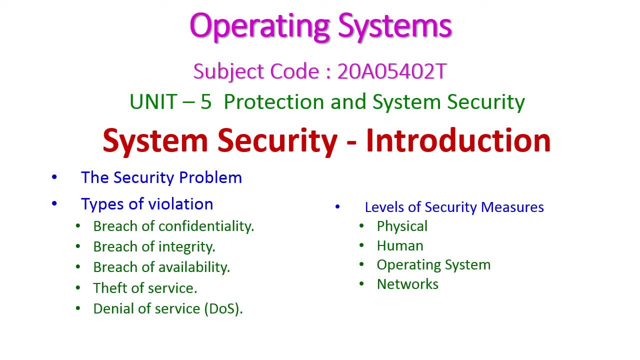 Hello friends, this operating system class we will start the second part of 50 unit, that is, system security, And let us see the introduction to system security in today's class And we will see the security problems and types of violations Here: breach of confidentiality, breach of integrity, breach of availability and theft of service, denial of service. So this will come under violations And after that we will see the levels of security measures. So the levels will be physical, human operating system and network level. These four will come under levels of security measures. 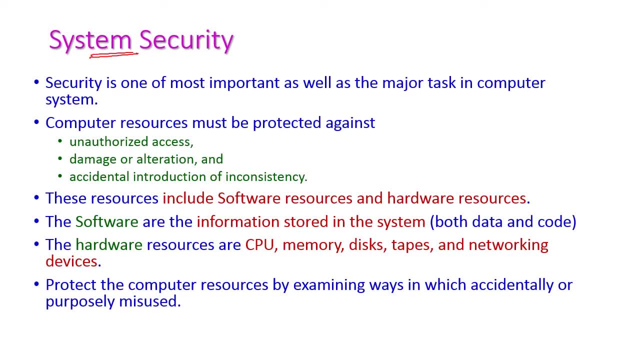 System security, which is nothing but our computer system security, And this is one of the most important as well as major task in the computer system. We have to protect our resources. Okay Now, the computer resources must be protected against unauthorized access, damage or alteration of resources and accidental introduction of inconsistency. So we have to protect our system from these things. 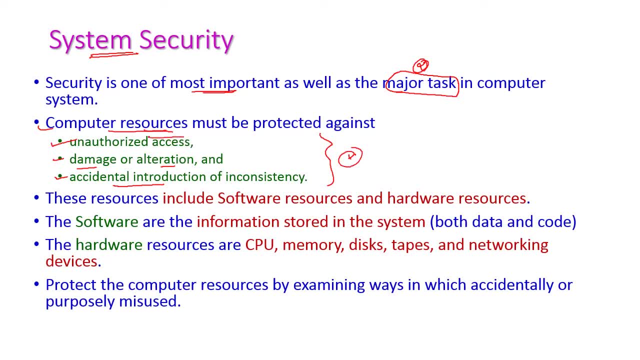 Okay, here the resources are nothing but Software resources as well as hardware resources. So we have to protect both software resources as well as hardware resources. Which are software resources? The information which are stored in our system. It may be either data or code, It may be system software, application software, whatever it may be, Okay. And when come to hardware resources, we are having CPU memory, that is, main memory disk, secondary storage, disk tapes and networking devices. 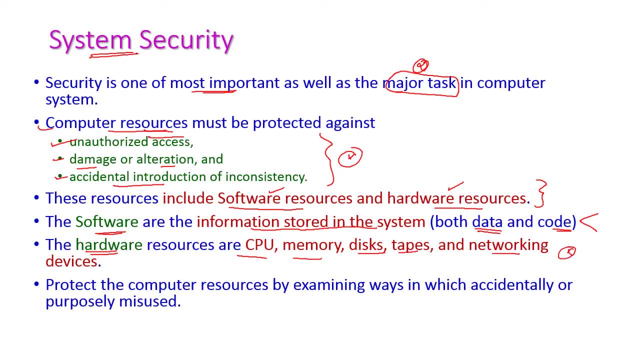 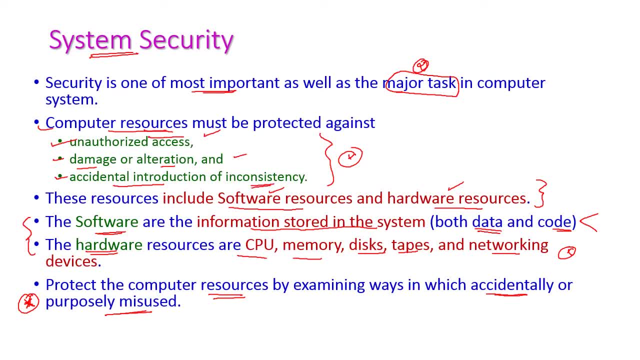 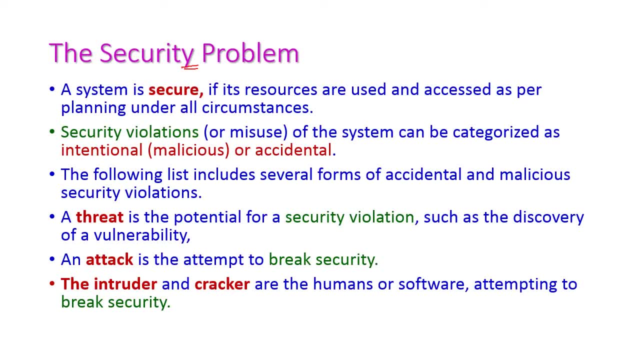 accidental introduction of inconsistency. so this is called as security, the security problems. when the system is secure, if the resources are used and access as per planning under all circumstance, then only the system will be called as a secured system. next, the security violations or misusing the system can be categorized as intentional misuse or accidental misuse. 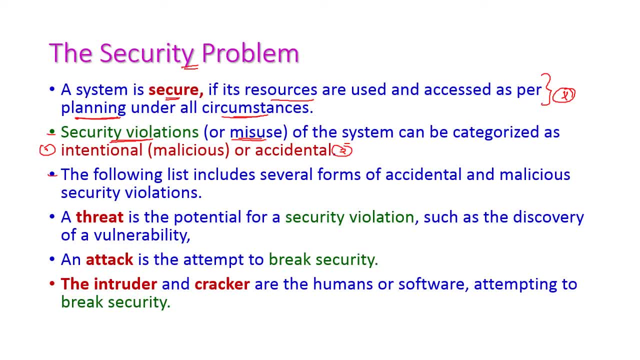 so two types okay here. the following list includes several form of accidental and malicious security violations. first one is threat. threat is a potential of security violations, such as the discovery of vulnerability. this is called as threat. threat is a potential of security violations, such as the discovery of vulnerability. this is called as threat. 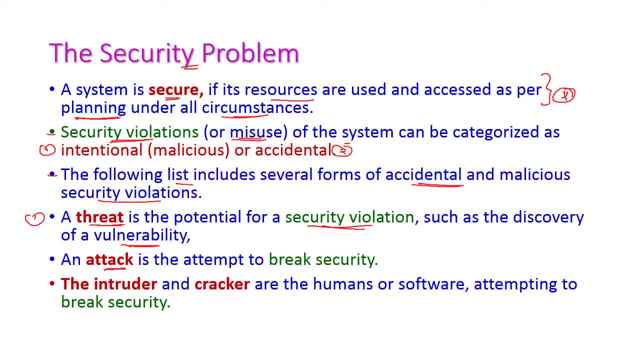 threat is a potential of security violations, such as the discovery of vulnerability. this is called as threat okay. and second one is attack. attacks is attempt to break the security. we are having some security measures. attack is nothing but breaking the security and the person. who are the intruders? 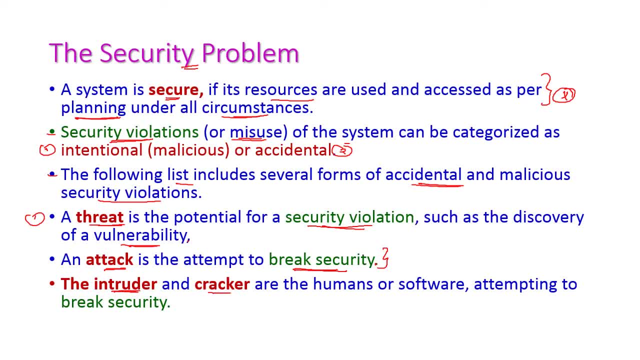 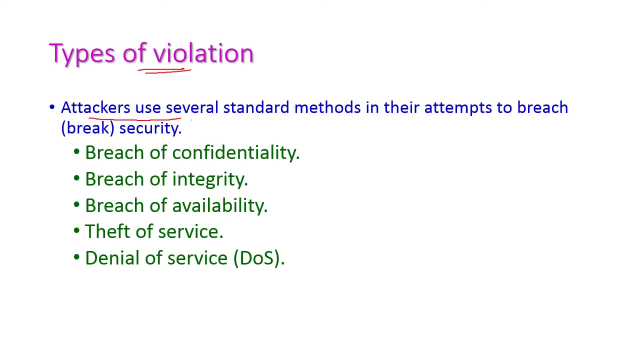 are crackers? okay, intruder or cracker are attempt to break the security, and these two persons may be humans or software. some software program may also act as intruder or cracker. right and next let us see the types of violations. attackers use several standard methods in their attempt to breach the security. bridge means break. 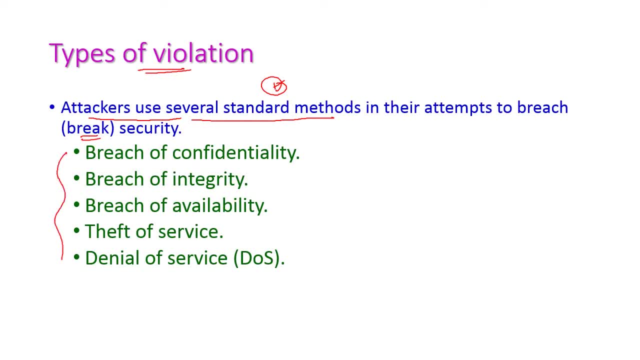 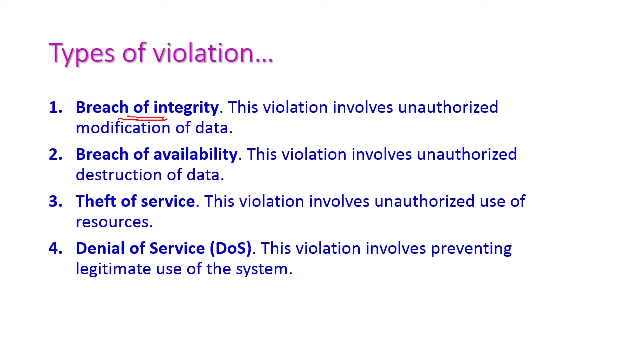 okay, here the different types are breaking the confidentality, breaking the integrity, breaking the availability and theft of services, denial of services. okay, so these are different types of violations. the first one is breach of integrity, that is, breaking the integrity. that means the violation involves unauthorized modification of data. okay, the data will be modified without the. 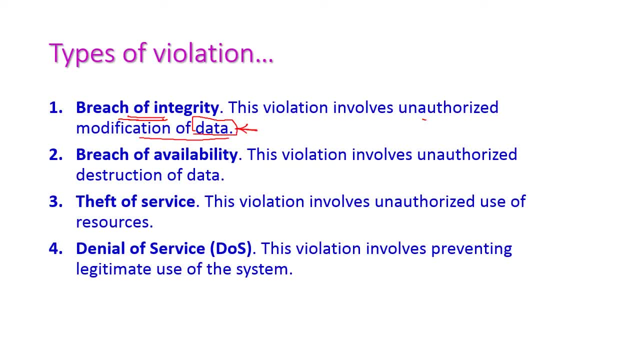 knowledge of owner. then this is called as breach of integrity. then breach of availability- this means an authorized destruction of data. the data will be deleted or modified without the knowledge of owner is called as breach of availability. and third one is theft of service. theft of service: that means unauthorized use of resources without the knowledge of owner, the resources will. 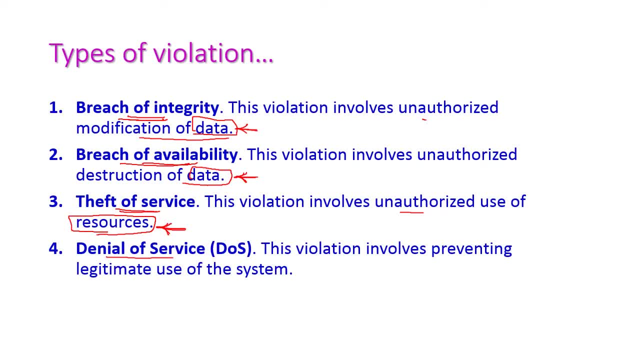 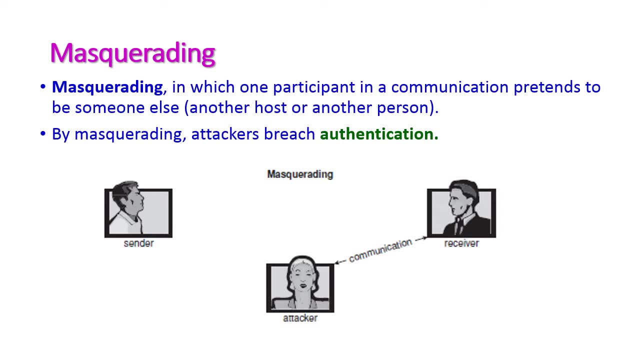 be misused. right and denial of service. this involves preventing legitimate use of the system That is called as denial of services. Apart from these four violations, some other are also there In this. first one is masquerading Here: one participant in a communication pretends to someone else. 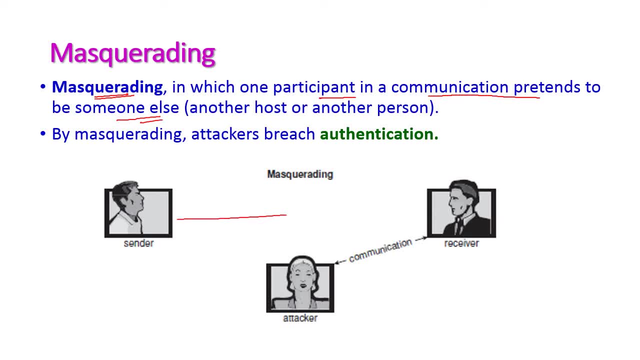 That is, the sender and receiver are communicating to each other Without the knowledge of sender. the receiver can give all information to the attacker also, So this is called as masquerading. By masquerading, attackers breach the authentication, So the authentication is broken in this masquerading attack. 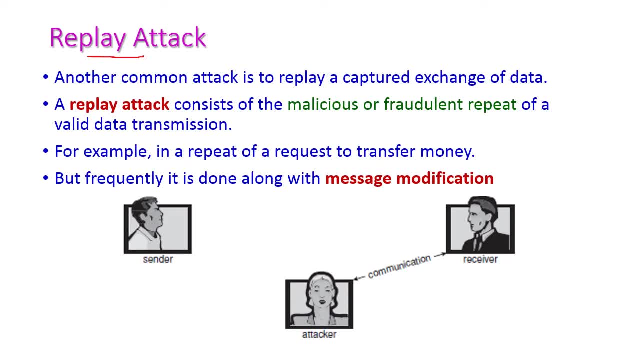 The second one is replay attack. That means replay, the captured exchange of data. What is that Replay attack, which consists of malicious or fraud and repeat of valid data transmission. The same valid data will be. the transaction will be repeated one more time. So this is one attack And, for example, in a repeat of request to transfer money. 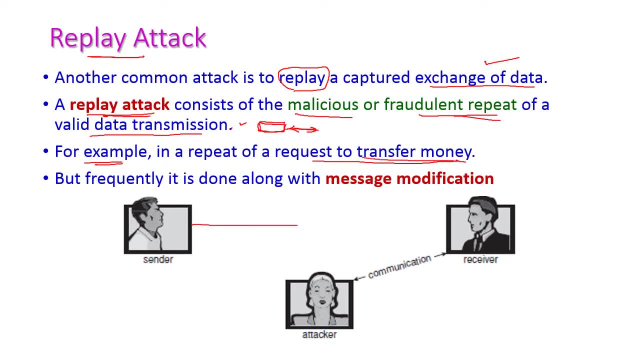 First, the sender and receiver are exchanging money. The sender requests money, for example 5000 rupees, from the receiver, and the receiver will give the same money to the sender. Now the attacker will receive the same message and the same message will be given to the receiver. 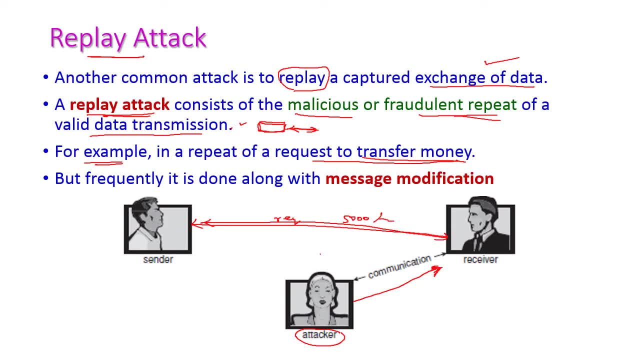 Now the receiver again transfers the same amount to the sender. That is, the receiver thought he is sending the amount to the sender, But the second time money will be received by the attacker. Okay, This is replay attack. Okay, But frequently it will be done with message modification. 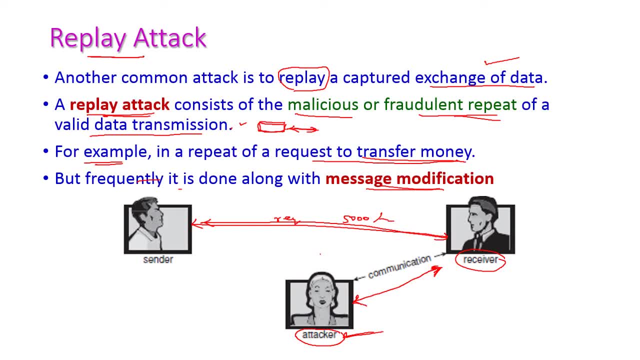 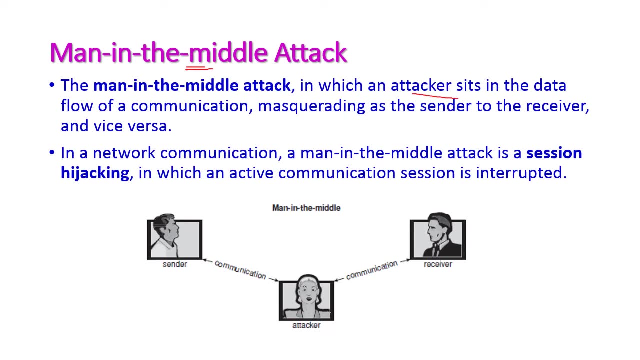 That is frequently. this attacker will send the same money request to the receiver and he will continuously get the money from the receiver. Both are possible. The next one is man in the middle attack. Here the attacker sits in the data flow of communication and mask reading as sender to receiver and vice versa. That means here the sender and receiver are actually communicating to each other. 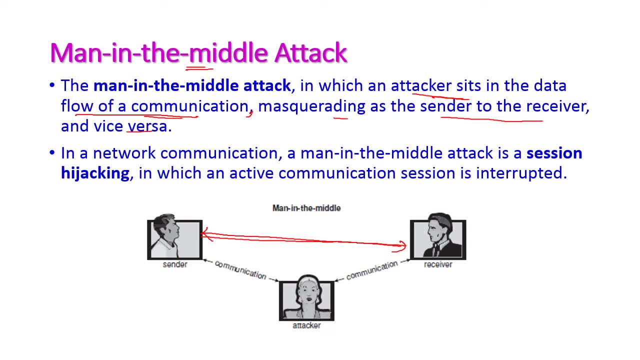 Okay, Now the attacker will sit in between the communication line. Okay, The attacker sits in between the communication line and the attacker will monitor both the communication from sender as well as the receiver. Okay, Here in network communication man in the middle attack is a session hijacking. It is called as session hijacking, in which the active communication session is interrupted. 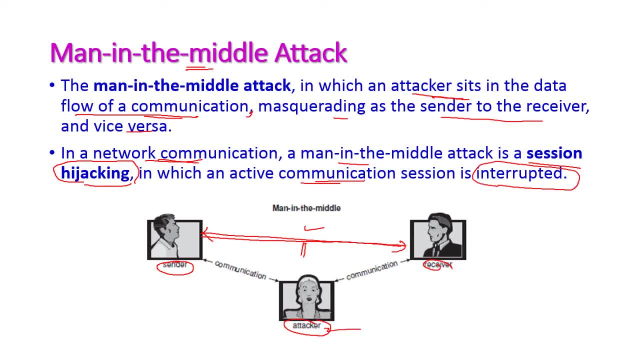 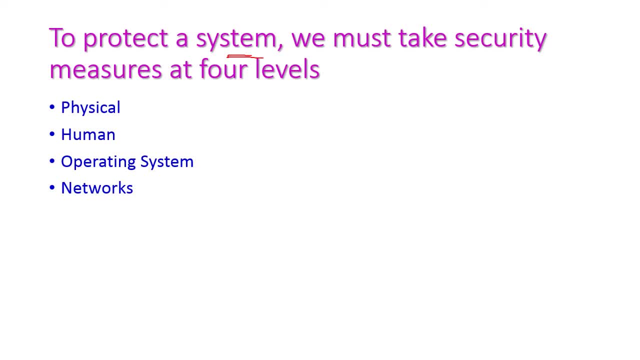 Because of the attacker who is sitting in the communication line. To protect a computer system, we must take security measures at four levels. Okay, These four levels are very important. First one is physical level and human level, operating system level and network level. 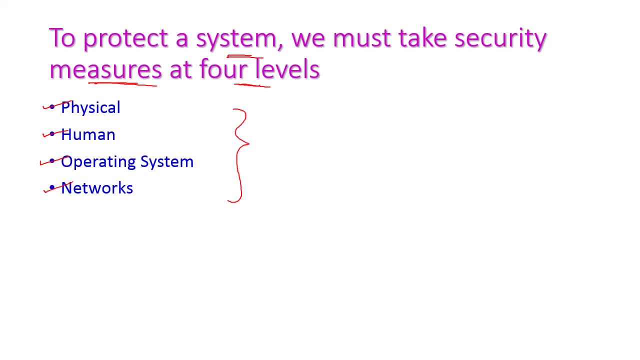 Let us see all these four levels in detail, one by one. The first one is physical level. Here the site is in front of the computer, Here the site is in the front of the computer And here the site is in the back of the computer. 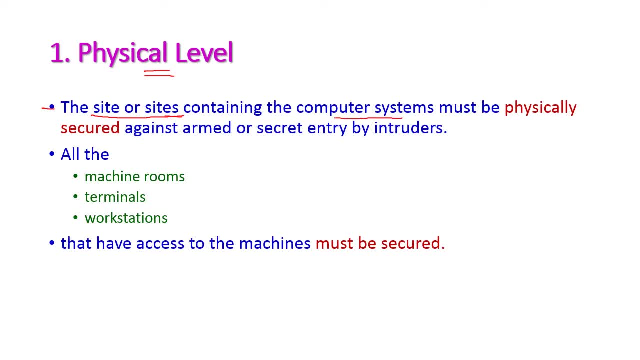 Site or sites containing the computer system. that means the data which contains the computer system must be physically secured against the armed or secret entry by the intruders. So we have to protect the system physically from the intruders. All the machine rooms, terminals, workstations that have accessed the machines must be secured. 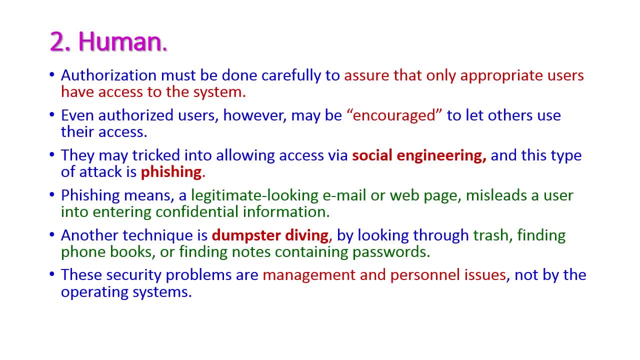 from the attackers. The second one is human: ie. authorization must be done carefully to assure that only appropriate users have accessed the system, ie only the authorized users have to access the particular systems. Sometimes the authorized users may allow the third persons to enter the system. 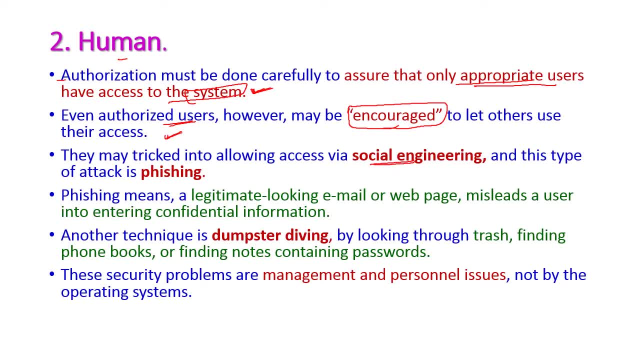 This is called as social engineering, ie The authorized user allow the third person to access the computer system is called as social engineering. So this type of attack is called as phishing Here the legitimate looking of email, ie the third person may access our confidential. 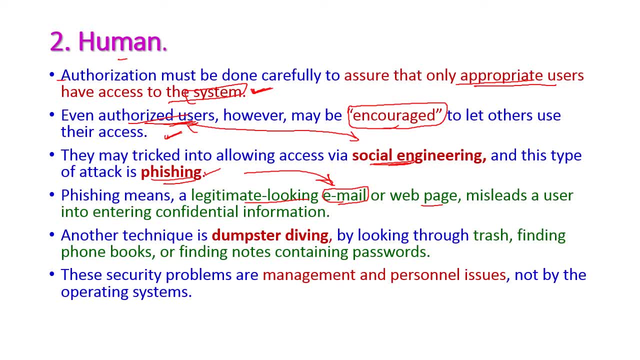 emails, web pages and enter into the confidential information without the knowledge of owner. the third person can access all those things. This is called as phishing. Another technique is dumpster diving, ie looking through trash, finding phone books, finding notes containing passwords. 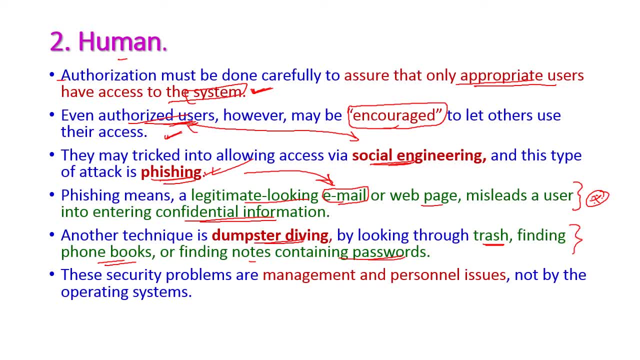 So the third person can access these things also. The security problems are management problem or personal issues. This is not under the operating system problem. That will not come under operating system problem. So this is actually the human problem. The third one is operating system. 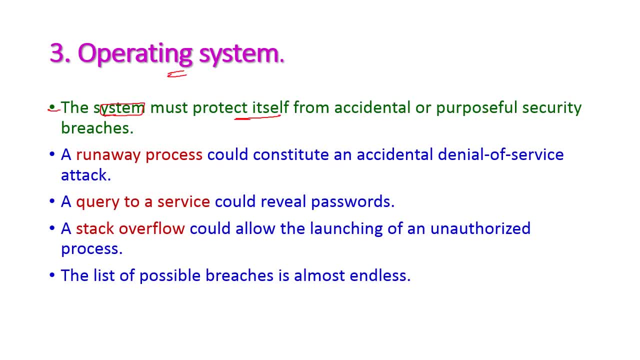 Here the computer system must protect by itself from accidental or purposeful security breaches. Here the runway process could constitute an accidental denial of service attack, ie DOS attack, and a query to a service could reveal the passwords and stack overflow could allow launching an unauthorized process. and this list of possible breaches. these are: 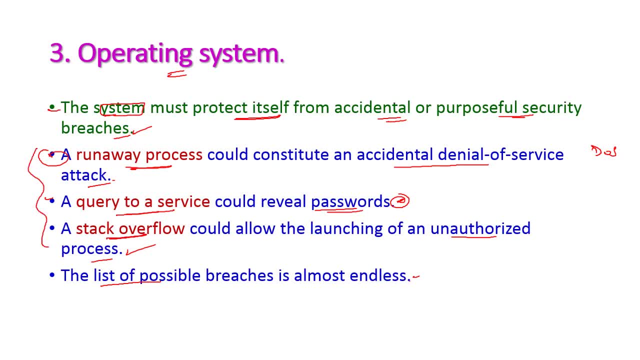 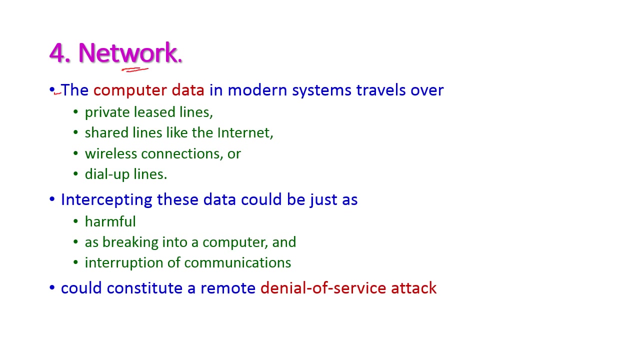 possible breaches is almost endless. which are the possible breaches? the runway process, query to a service, stack overflow, likewise, so many other process are also there, and this is almost endless. These are the problems by operating system. And the fourth one is network. Here the computers will be connected to each other over a network, over a network, hence. 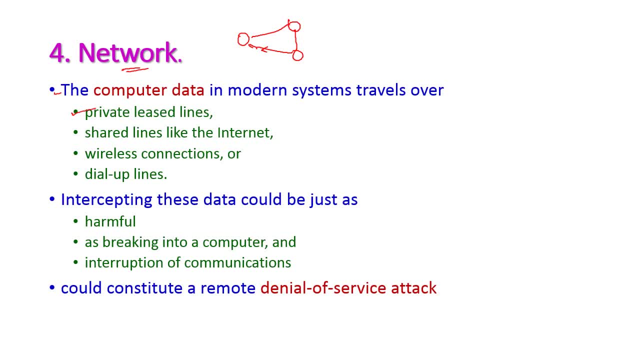 the data will be traveled over the private list line, shared line, like the internet, wireless connections or dial up lines. so by using all these lines, we can connect our computers. hence the data will be transmitted through these lines, and intercepting data could be just as harmful.